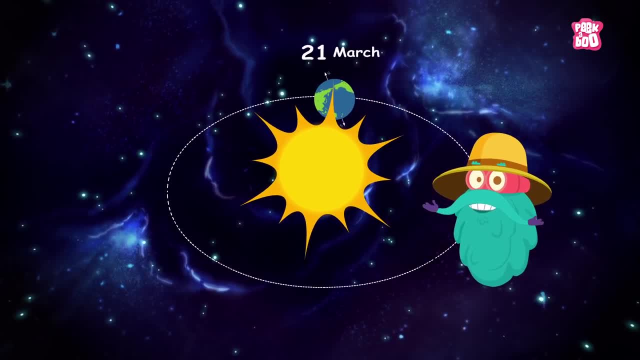 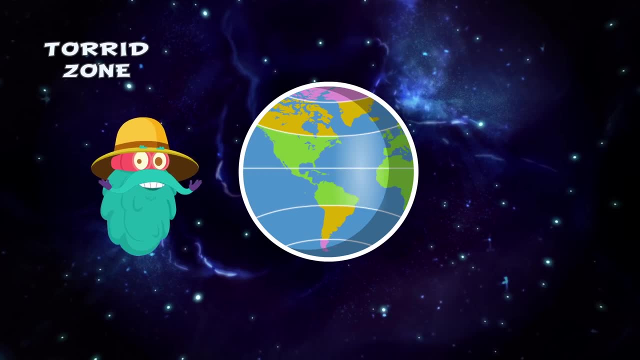 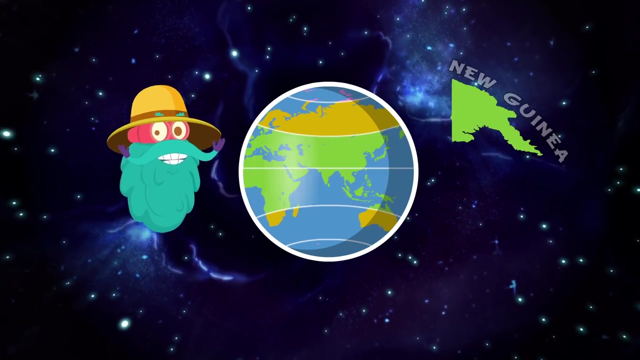 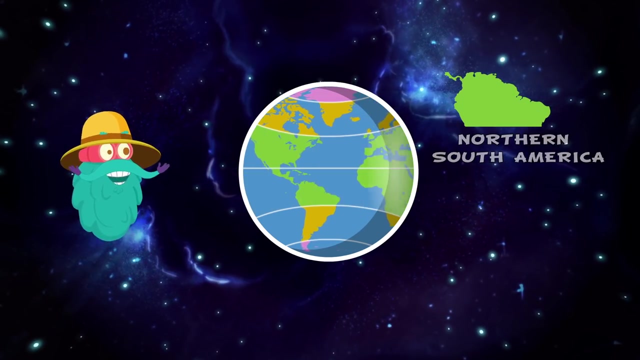 Mark the dates again. It usually happens on March 21st and September 23rd. The Torrid Zone includes most of Africa, Southern India, Southern Asia, Indonesia, New Guinea, Northern Australia, Southern Mexico, Central America and Northern South America. 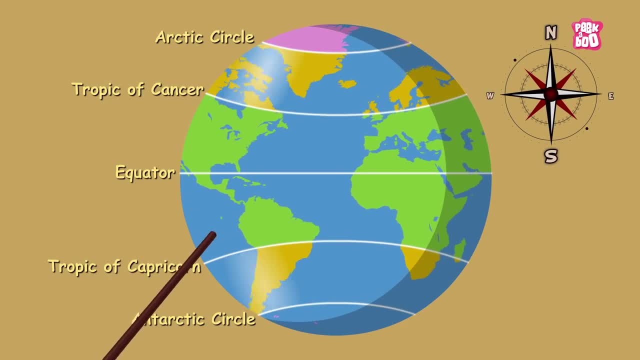 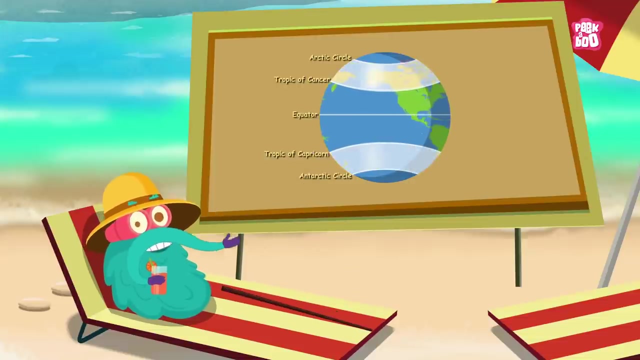 Next is the Temperate Zones which fall between the two tropics and the Arctic Circle in the north and the Antarctic Circle in the south, respectively. This is the perfect vacation zone, as it usually has mild temperatures and enjoys all the four seasons annually. 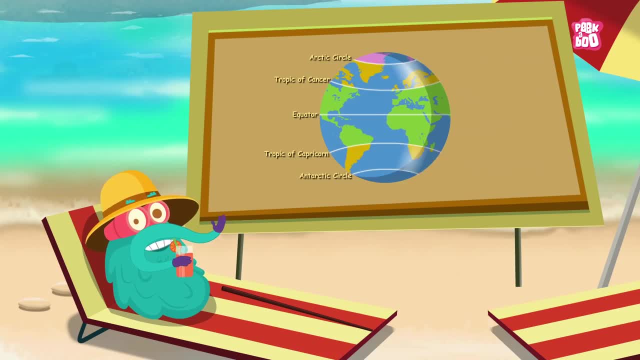 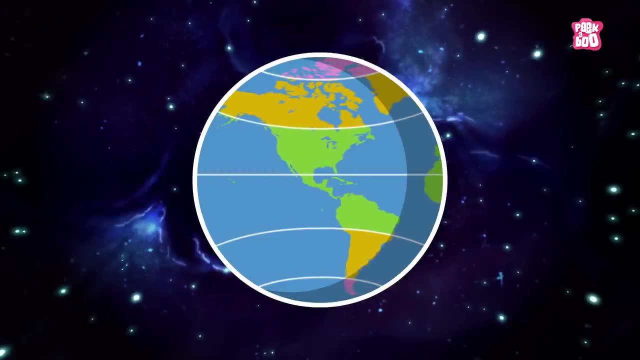 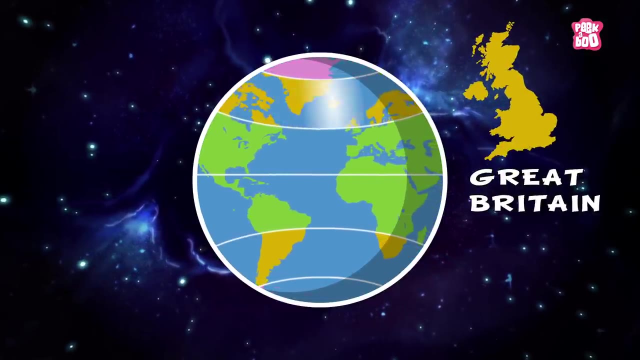 Summer, Spring, Autumn and Winter. This is because in these regions the sun is never directly overhead. These are the regions that fall in the Temperate Zone. The North Temperate Zone includes Great Britain, Europe, Northern Asia, North America and Northern Mexico. 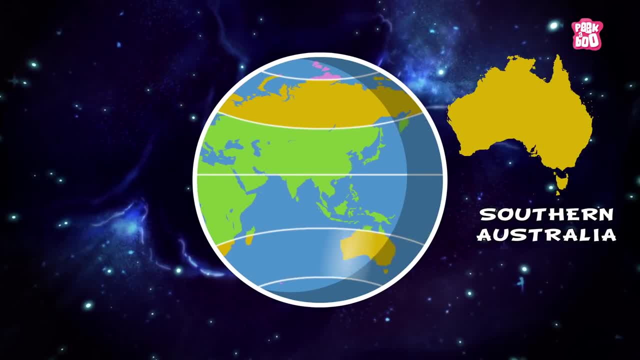 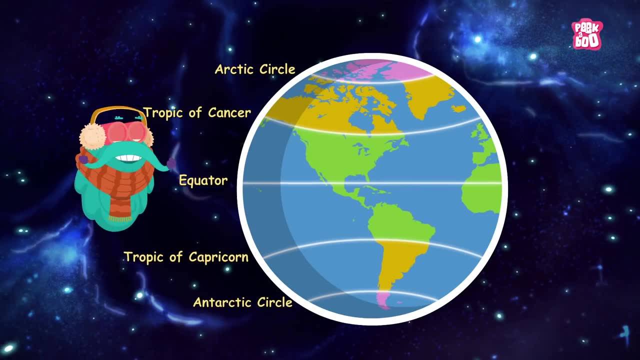 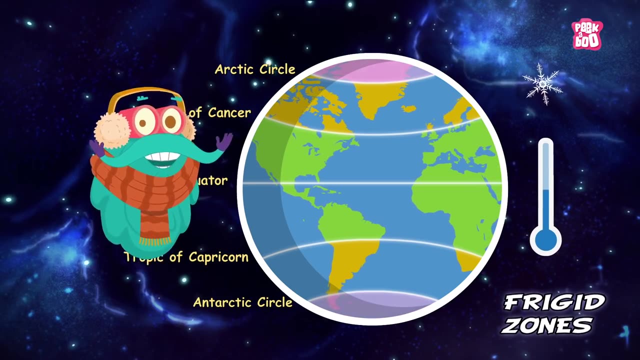 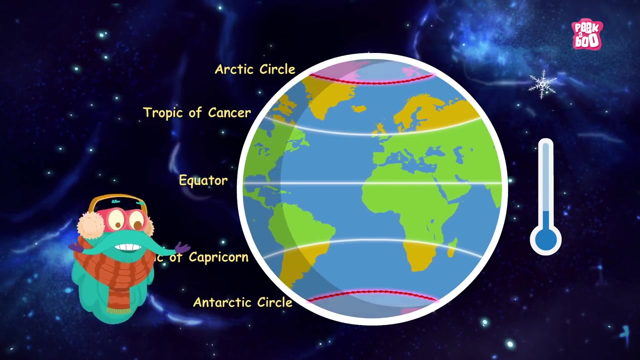 The South Temperate Zone includes Southern Australia, New Zealand, Southern South America and South Africa. The last of the zones is the other extreme, and so is called the Frigid Zones. It is the coldest part of the planet. These zones lie beyond the Arctic and the Antarctic Circles. 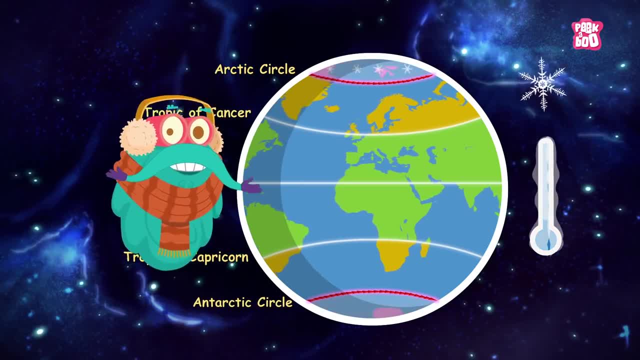 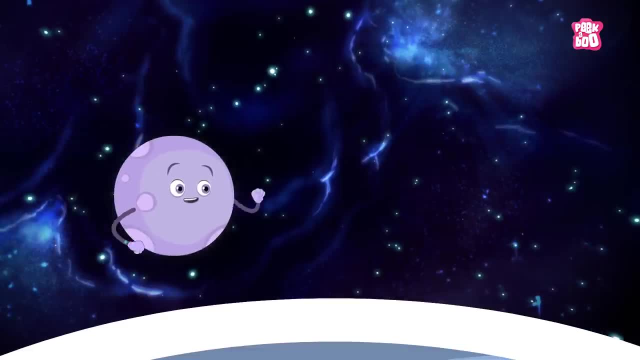 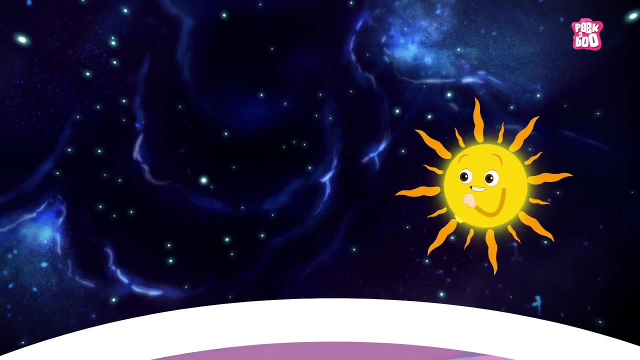 So you know they are freezing, Haha. And even their day and night cycles are super weird, That's right. Sometimes the sun doesn't rise or set for 24 hours and sometimes the day is literally one year long, with 6 months of daylight and 6 months of night. 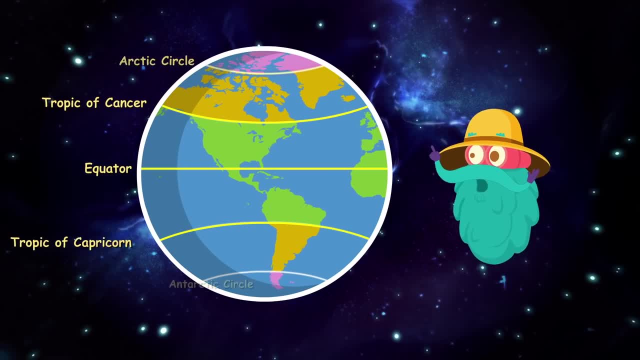 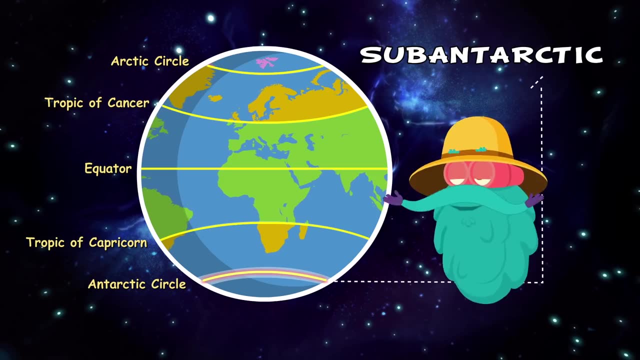 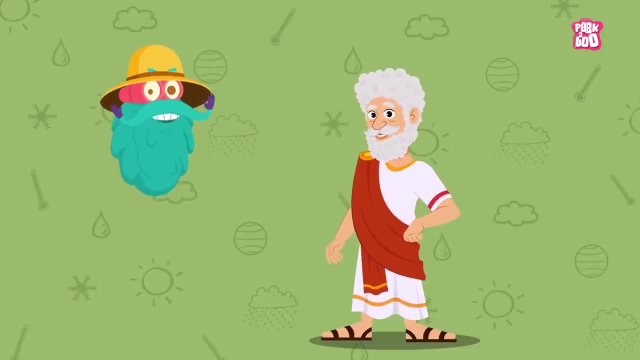 Trivia Time. The edges of the Temperate Zones are also sometimes referred to as the Sub-Tropics, Sub-Arctic and Sub-Antarctic. Aristotle, the ancient Greek scholar, was the first one to come up with the idea of Climate Zones. 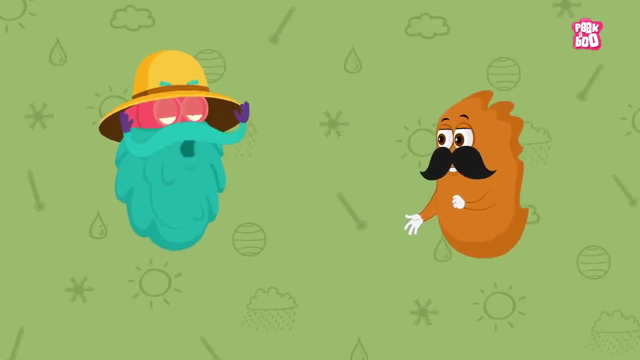 Well, friends, now you have a better idea of how the climate of our planet works, And seeing how the climates are getting all topsy-turvy these days, you know where it might be going wrong. So tune in next time for more fun facts.